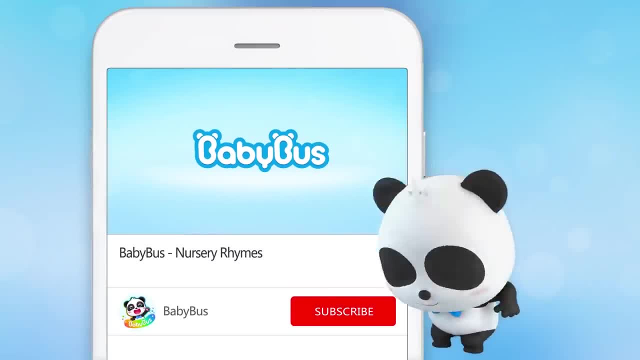 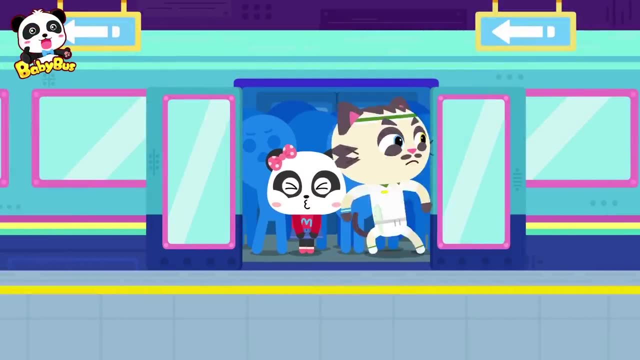 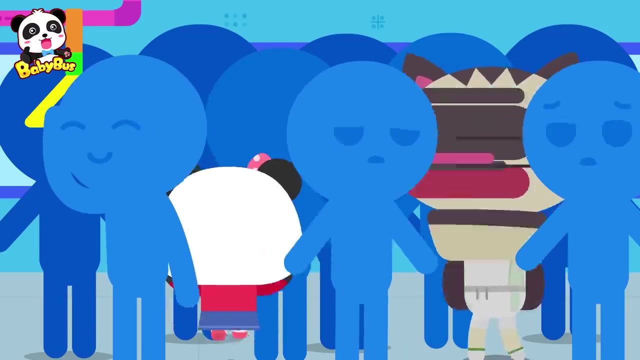 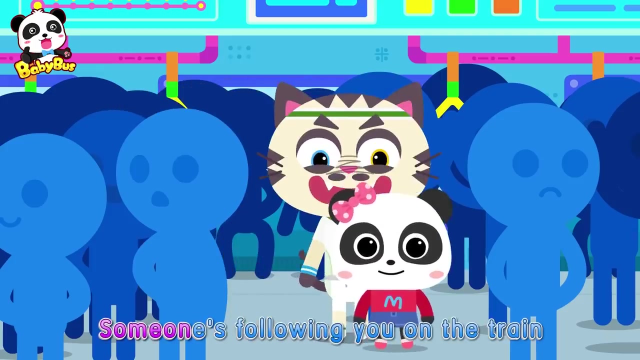 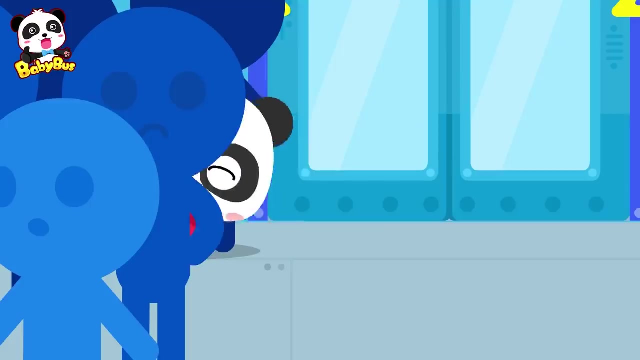 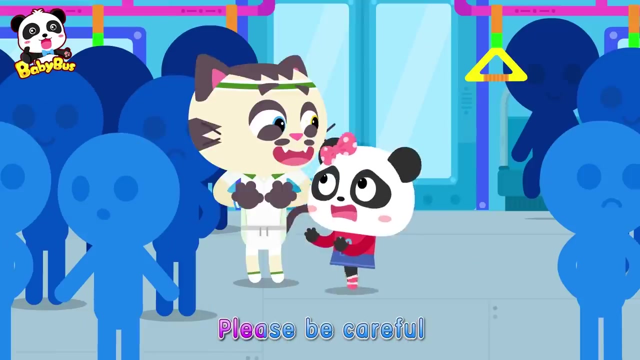 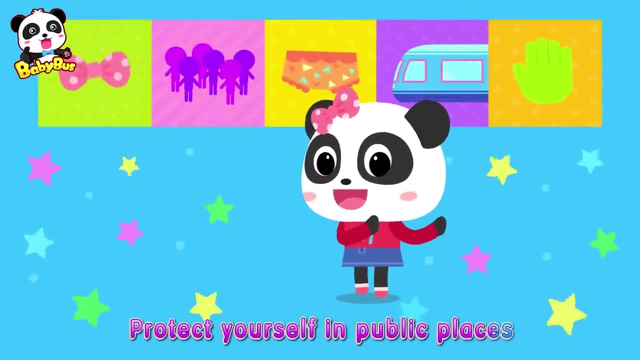 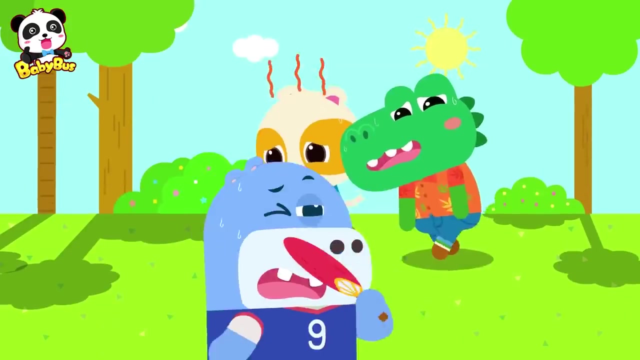 Baby Bus. Click here to subscribe. Someone's following you on the train. Someone's following you on the train. A shadow behind you, please be careful. A shadow behind you, please be careful. Go away, Protect yourself in public places. Keep your private parts safe. Don't forget to subscribe. 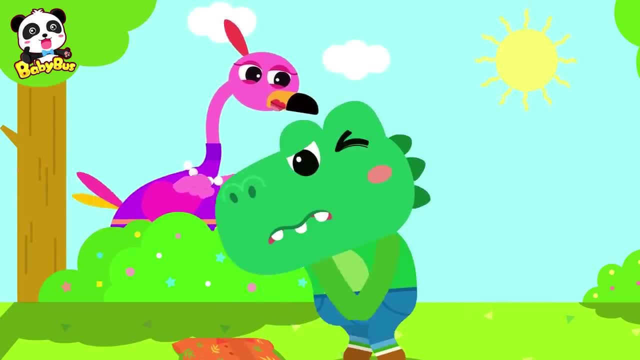 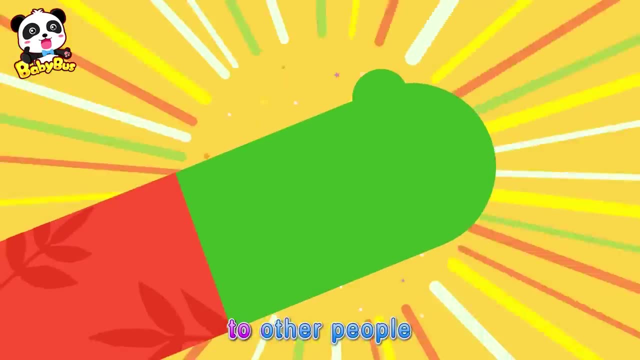 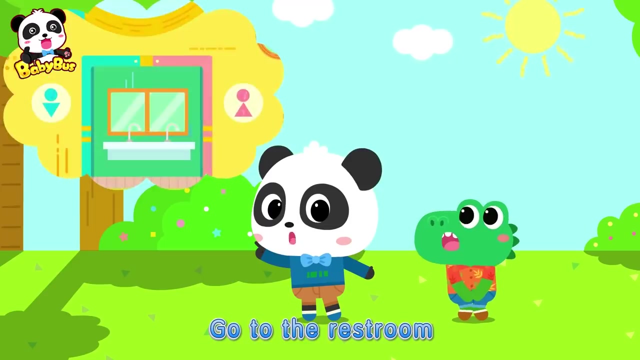 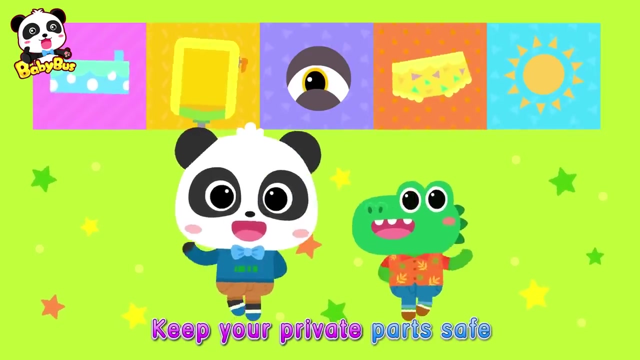 Don't take off your clothes in public places. Don't take off your clothes in public places. Don't show your private parts to other people. Don't show your private parts to other people. Go to the restroom. Protect yourself in public places. Keep your private parts safe. 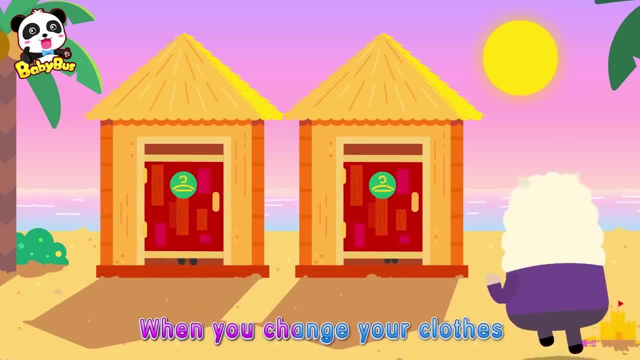 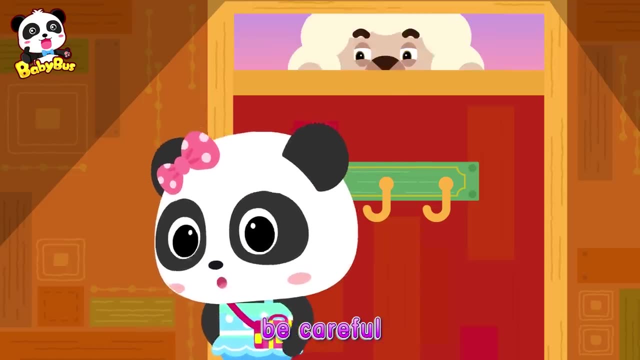 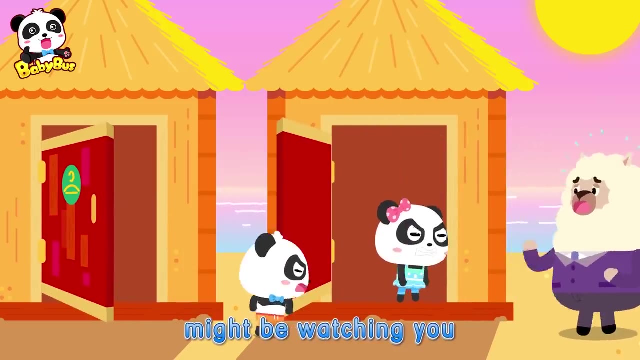 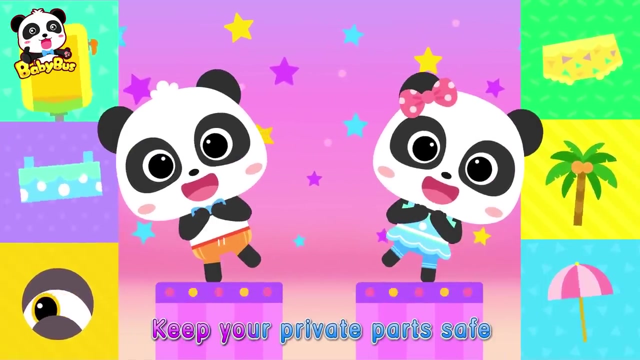 When you change your clothes, be careful. When you change your clothes, be careful. Someone's big eyes might be watching you. Someone's big eyes might be watching you. Protect yourself in public places. Keep your private parts safe. Keep your private parts safe. Always keep your private parts safe. 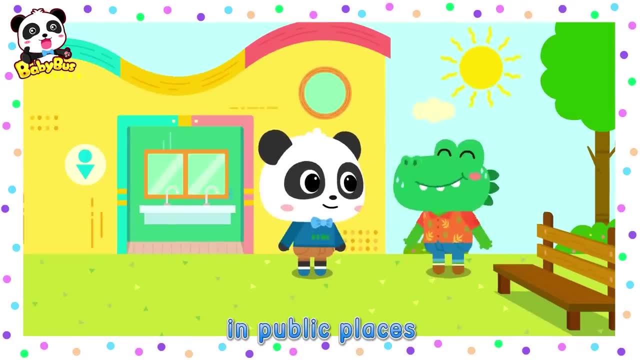 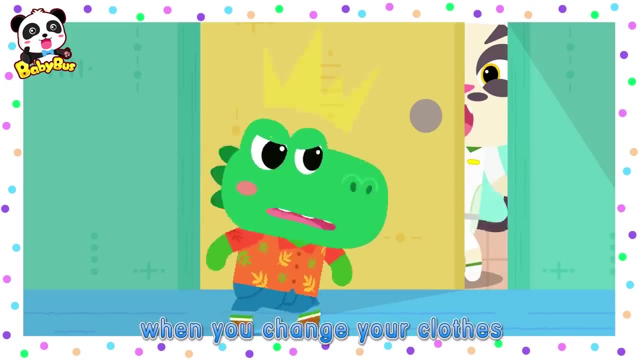 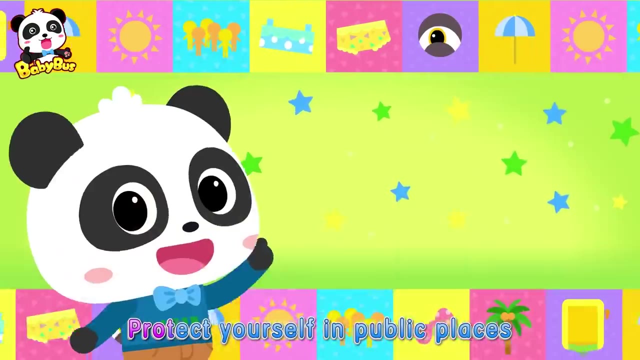 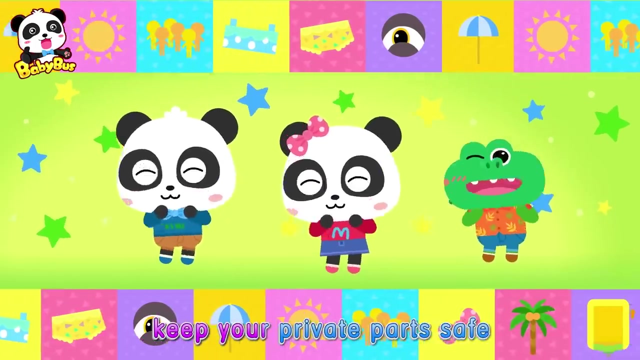 Always keep your private parts safe, Private parts covered. in public places. If you notice that someone is trying to touch you or is watching you when you change your clothes, shout out loud, Go away. Go away. Protect yourself in public places. You need to keep your private parts safe. For more information, visit wwwfemaorg.